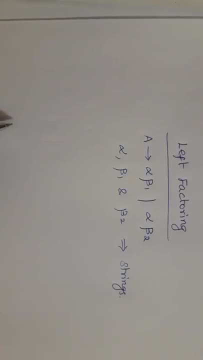 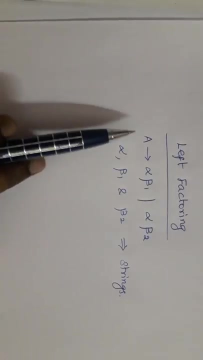 Hello everyone, in this video we are going to see about left factoring. So when two or more productions are starting with the same set of symbols, then we will get confusion like which of the two productions to be used to expand the non-terminal A, So whether the non-terminal A can. 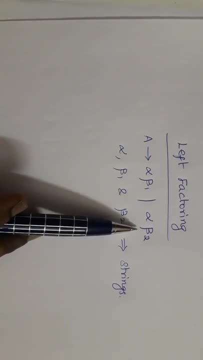 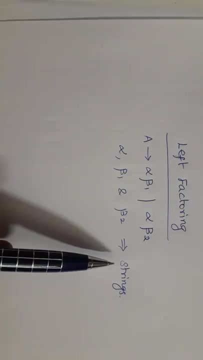 be replaced by using the first production or the second production, because both the productions are starting with the same string. Here alpha, beta 1 and beta 2 are strings, So that we need to do a grammar transformation called left factoring. Left factoring is a grammar transformation used. 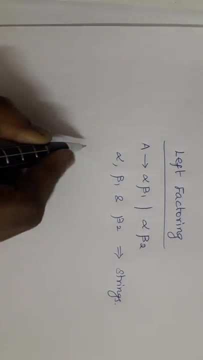 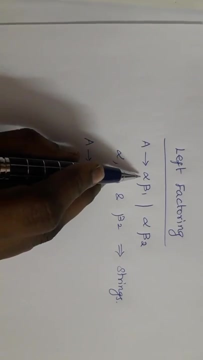 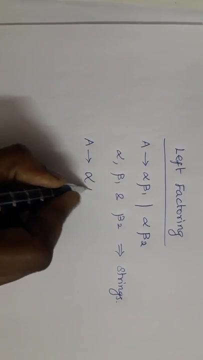 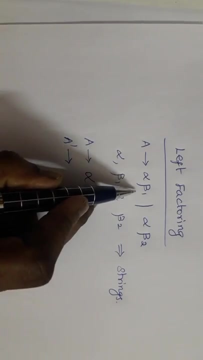 to avoid this confusion. So the general syntax is: A tends to this non-terminal A tends to. First we need to write all the common symbols from the productions. So here, in these two productions, alpha is a common symbol, So alpha, a new symbol, A dash. Then this A dash implies the remaining symbols from the. 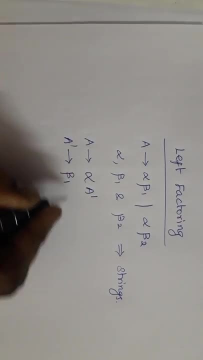 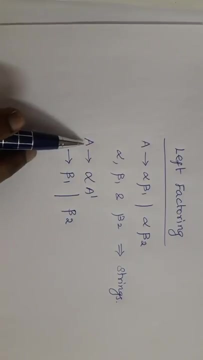 productions. So from the first production beta 1 is a remaining symbols because it is a string. then beta 2.. So here, initially A is expanded till alpha, all the symbols in alpha, Then the remaining symbols. based on the remaining symbols, A dash can replace either beta 1. 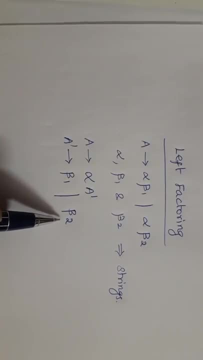 or beta 2.. So here A dash can replace either beta 1 or beta 2.. So here A dash can replace either beta. you can use beta 3 or beta 2, you can use yebda or beta 2.. Here so the confusion is eliminated. 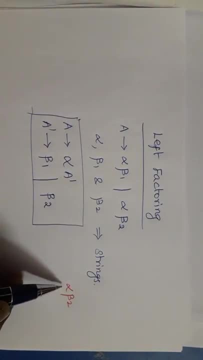 For example, if we want to construct a parsery for alpha beta 2. We need to start with. the start symbol of the grammat A can be expanded by using this production: alpha beta, sorry, alpha a dash. then this a dash can be replaced by using: 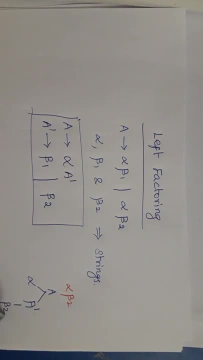 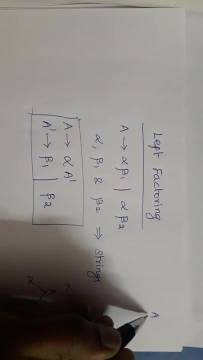 this production or this, but we need beta 2, so a dash can be replaced by this b2 here, but before left factoring, if you start constructing parse remains. a can be replaced by: we don't know whether to whether we have to use this production or this production to retrieve this, because we 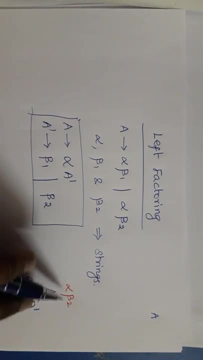 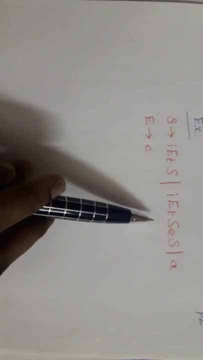 know about only alpha. we don't know about the second symbol, beta2. so, in order to avoid the confusion, left factoring is a grammar transformation. top down parsing for the top down parsing, left factoring is a useful transformation. now consider this example. it's a. it is a well-known grammar. 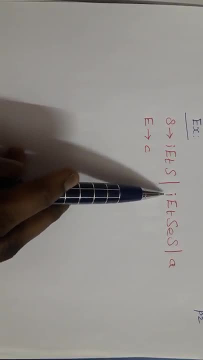 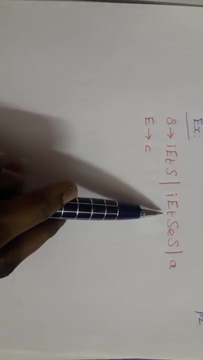 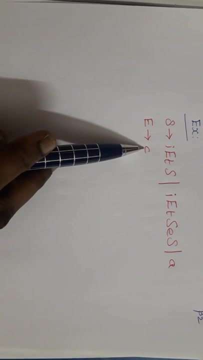 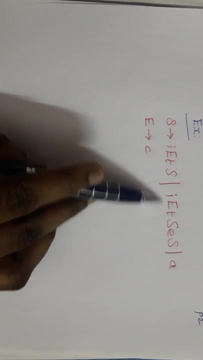 called statement tends to: if expression, then statement. if expression, then statement, l statement. this is a if if, then statement. this production is for: if, then l statement, then a normal a, then this expression may be any condition. so e tends to so. here the two productions are starting with the common symbols: iets, iets. so we need to do. 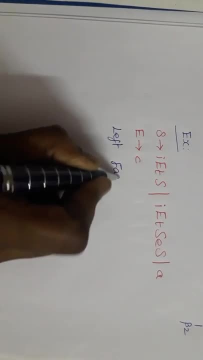 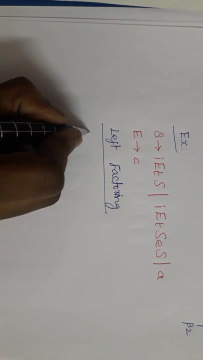 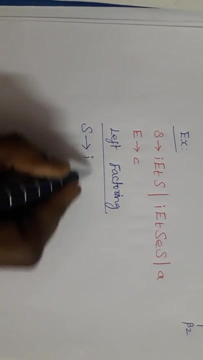 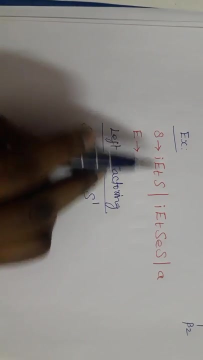 left factoring for this grammar. so to do the left factoring first, we need to write: yes, write all the common symbols from the productions. so i e t s, then a new symbol is dash. there is no change with. s tends to a, because here it's a separate production. 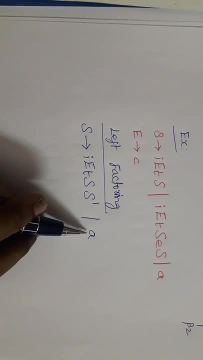 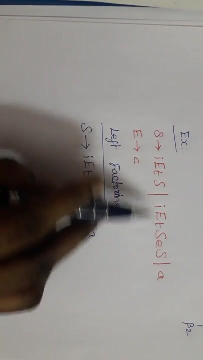 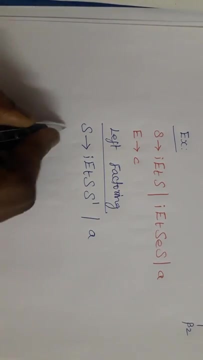 it is not starting with the common symbol. so don't change, don't do any transformation in this production. so s tends to. a is written as it is. we need to do the left factoring for this production, only so these two productions only. so s tends to i e t s s dash, then this s dash tends to. 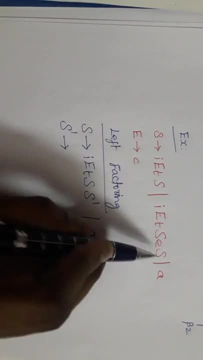 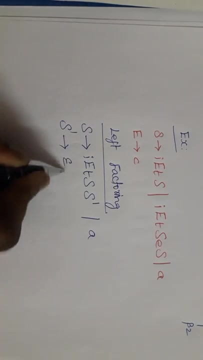 to something b dot z dash. here the component is denant with s, and we can divide agents into a, b and a – d, so a a s going ahead s Roman formikk i s it's not s bar, so a a na na. it's not a dso just a normal sound. 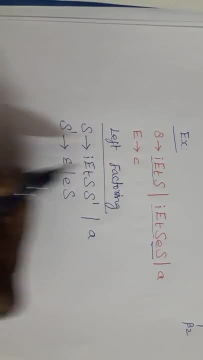 Fait Xiao. so these four symbols are followed by epsilon actually. so epsilon barhere e s. so the common symbols are: here iets, here ieds. so when we write the remaining symbols here, we need to consider epsilon and here estate. then there is no change in E production. 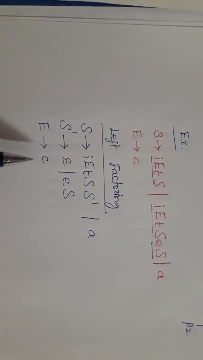 so E tends to c, C. So we have done left factoring for this grammar, Thank you,